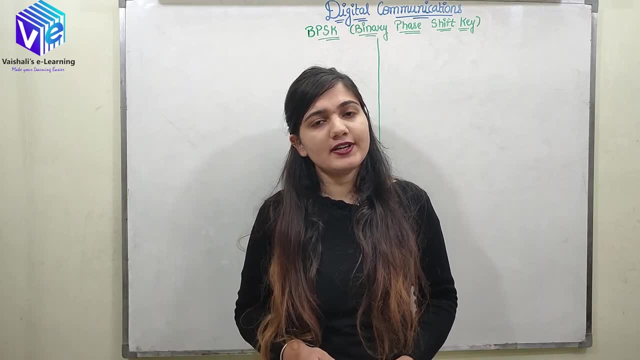 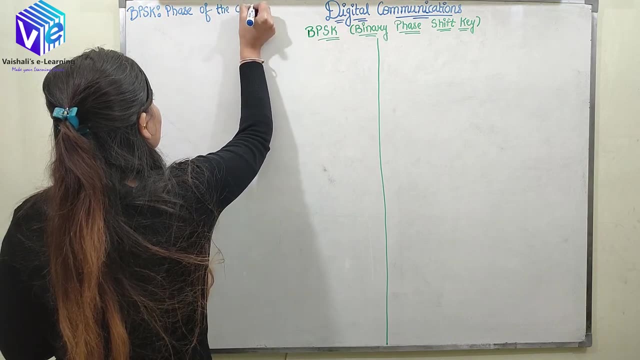 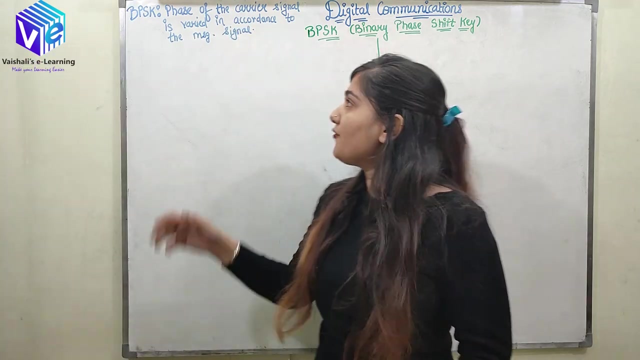 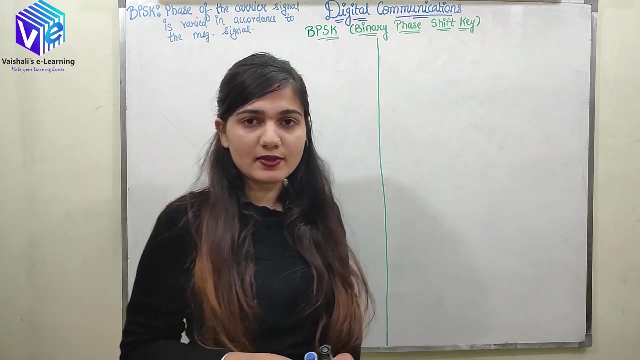 In the receiving block diagram we will see the coherent and non coherent type of receivers. So let's begin. So here, phase of the carrier signal is changed in accordance to the message signal. So let's understand this with the help of an example. So I am taking a digital. 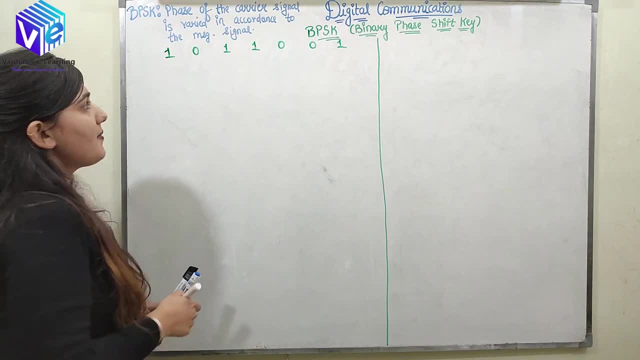 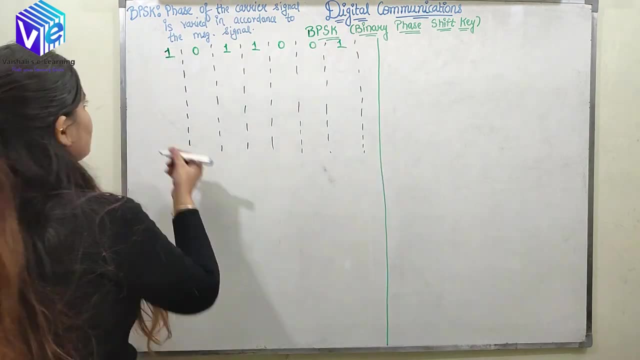 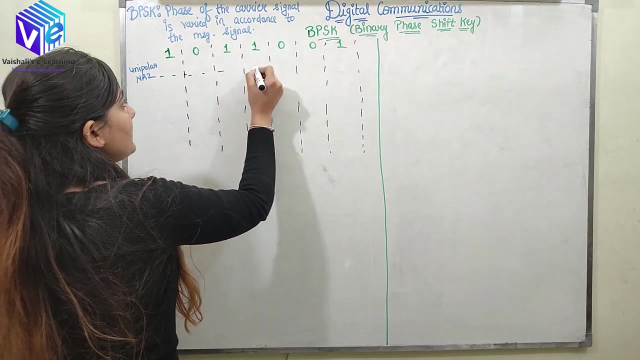 data. So I am taking this example. My digital data is this: So if I have to represent my digital data in unipolar NRZ format, I know that 0 is represented by 0 and 1 is represented by plus V voltage. 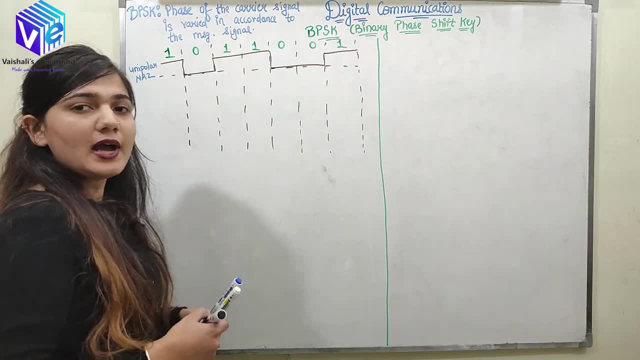 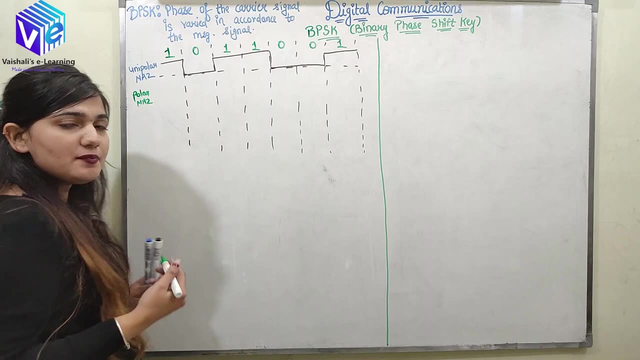 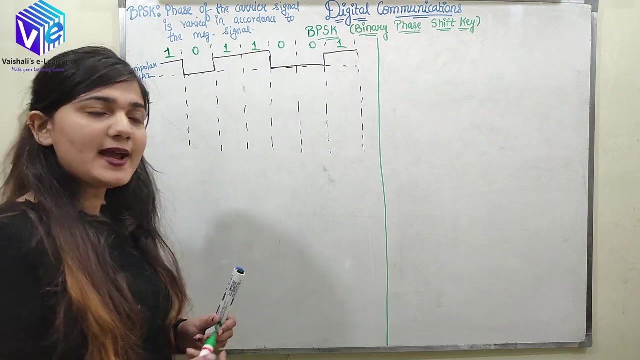 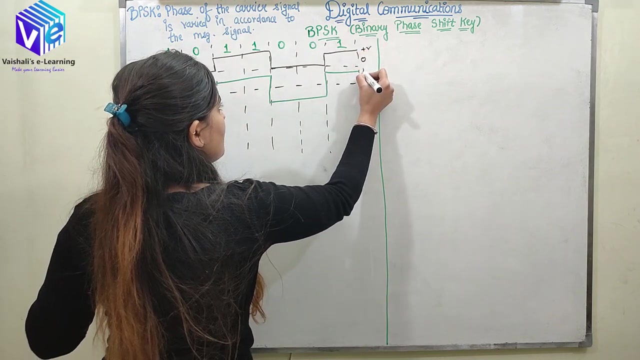 So now I will convert this unipolar NRZ data into the polar NRZ data. So now in polar NRZ I know 1 is represented by plus V voltage and 0 is represented by minus V voltage. So here I had plus V 0, plus V 0, minus V. So now I hope you understand what is a unipolar. 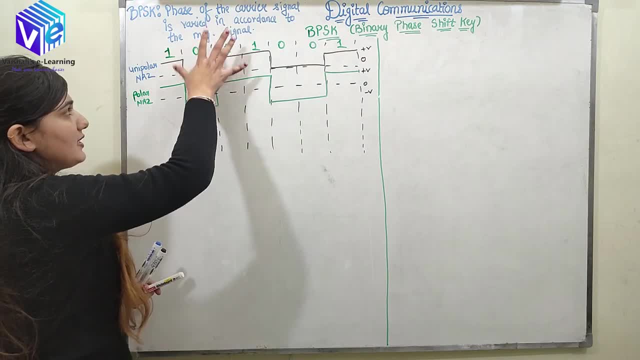 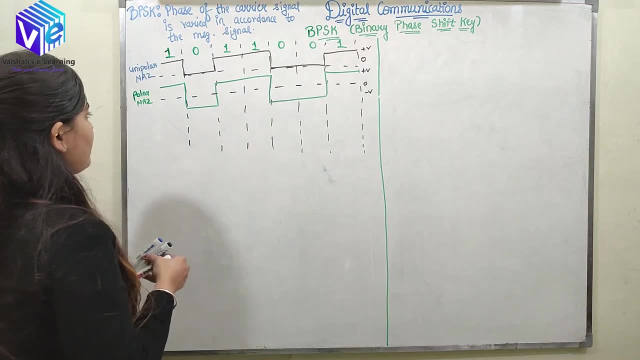 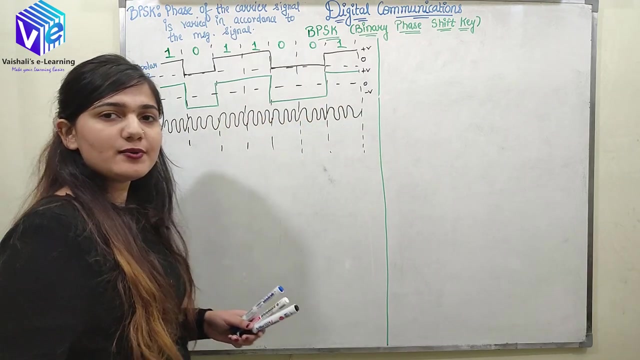 and polar difference. So I converted this unipolar NRZ format into polar NRZ format. Now I will take a carrier signal which is high frequency, So this is my high frequency carrier signal. So if I multiply this polar NRZ format with 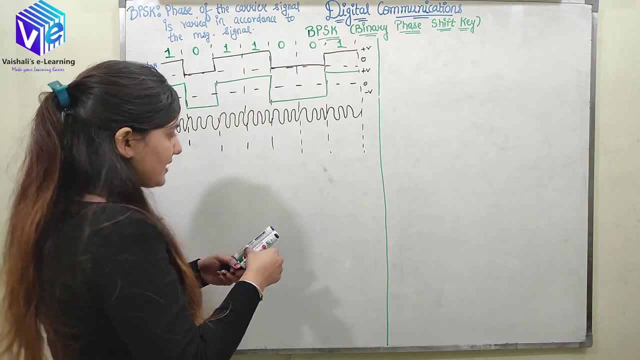 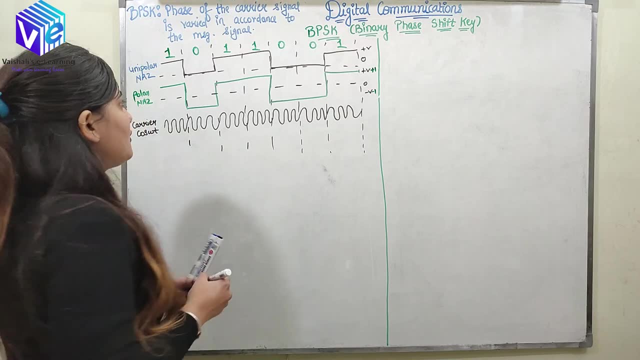 this high frequency carrier signal. So here I am taking a generalized case where I am taking the plus V voltage as plus 1 and minus V voltage as minus 1.. So at 1 it is represented by plus 1, and at 0 it is represented by minus 1.. So now, when I multiply the polar NRZ format: 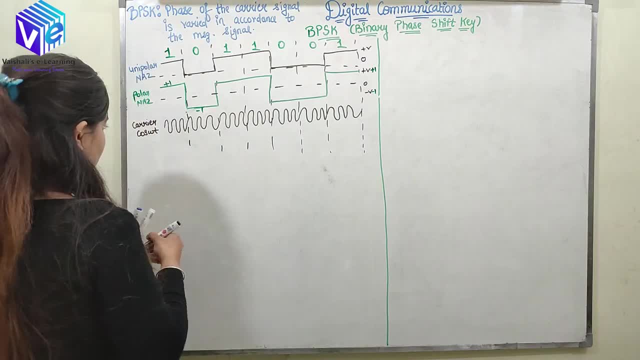 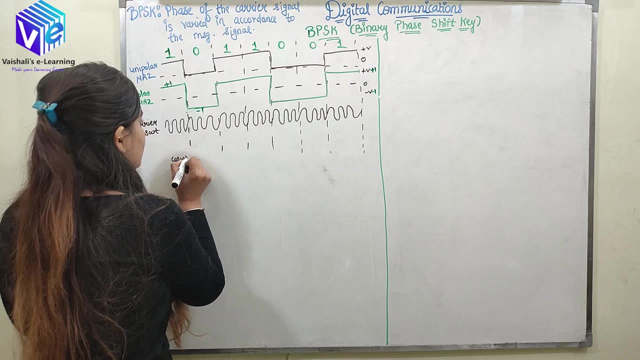 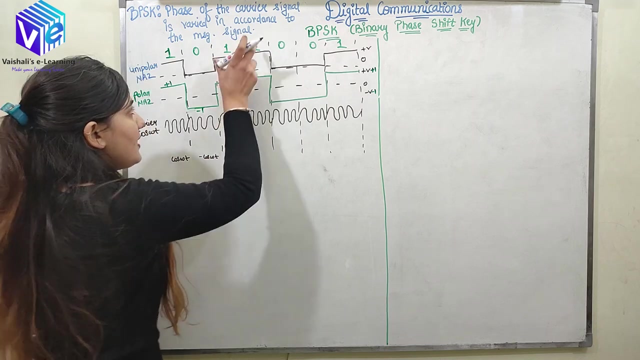 with the carrier signal. So here, when I have 1,, 1 is multiplied by cos omega t, I will get cos omega t. So when I have 0, here minus 1 is multiplied by cos omega t, I will get minus cos omega t. Here 1 is multiplied by cos omega t, Again I will get cos omega t. 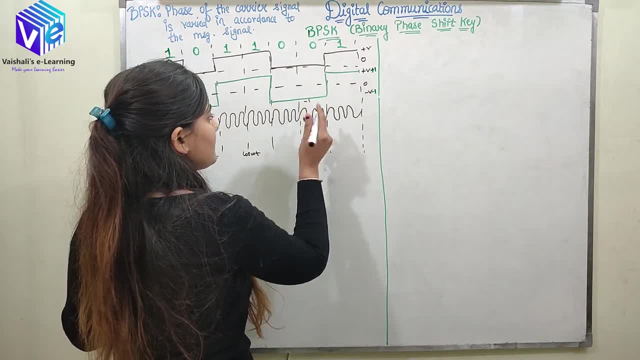 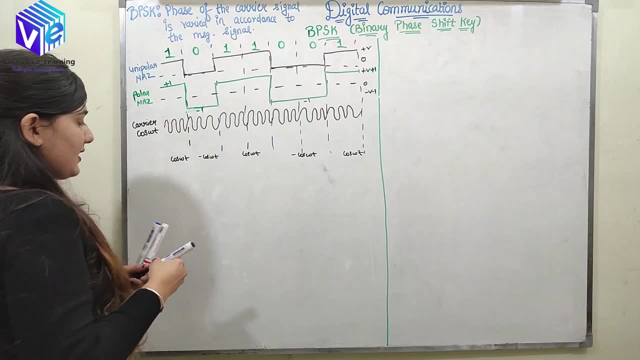 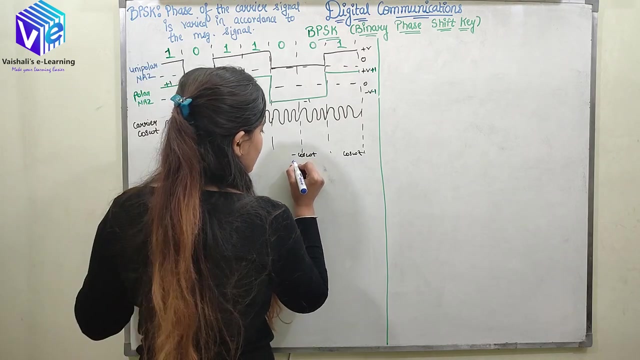 Here 0 is multiplied by cos omega t. So which means minus 1 is multiplied by cos omega t, I will get minus cos omega t, Again cos omega t. So now I can represent my minus cos omega t as cos omega t plus pi, Similarly here. So now when I have 1, I have cos omega t. 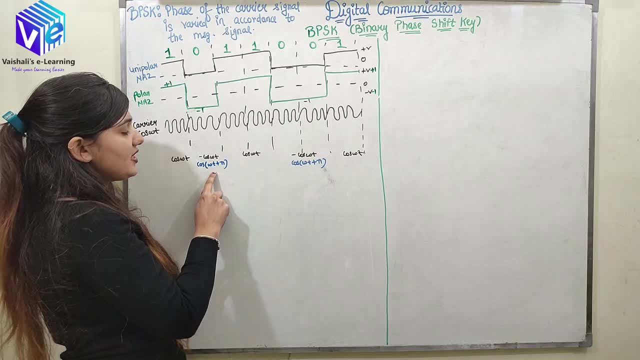 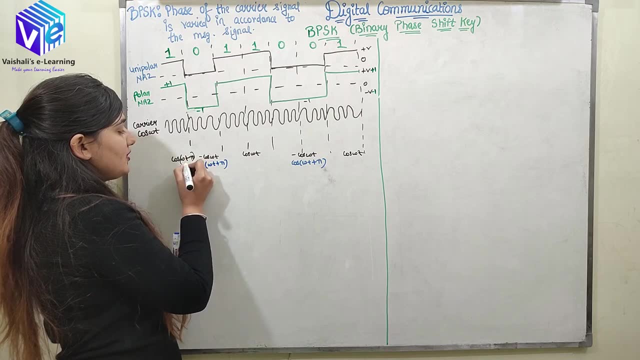 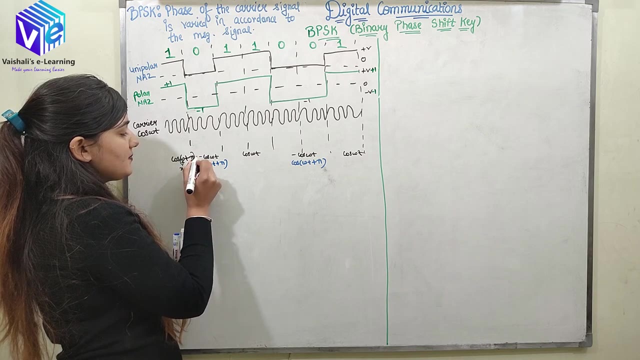 When I have 0,, my phase changed to cos omega, t plus pi. So here the phase is represented as plus 0. So this is my frequency, Omega represents my frequency, t represents my time and plus anything represents my phase. So here I have plus 0, here I have plus pi. 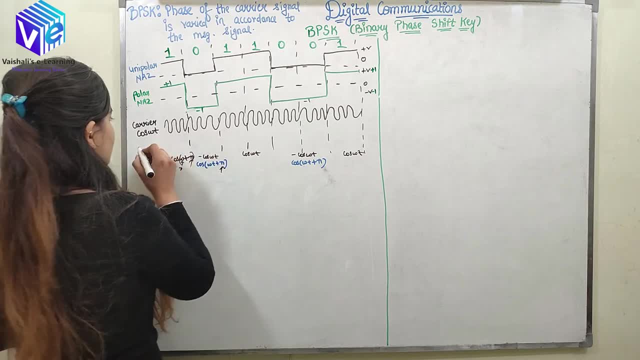 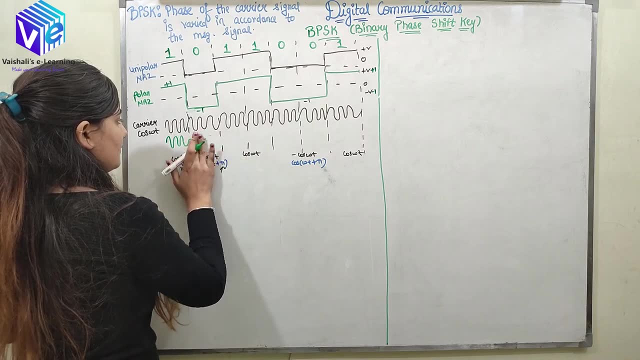 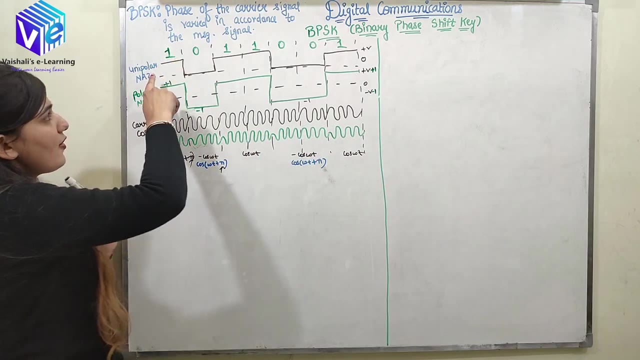 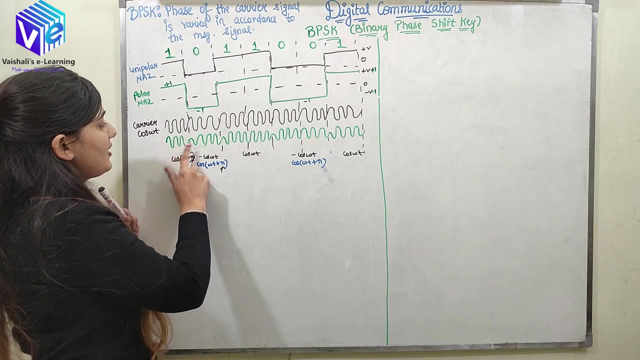 So phase changed from 0 to pi. So now the output modulated signal is represented like this. So whenever I have the transition from 1 to 0 or 0 to 1, I have pi shift in the phase. So when I have transition from 1 to 0, here the phase was shifted Again. when I have transition, 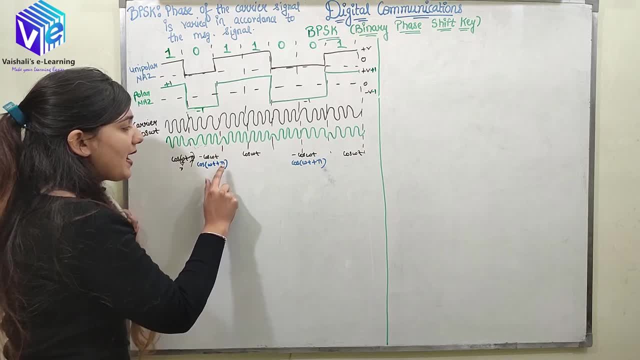 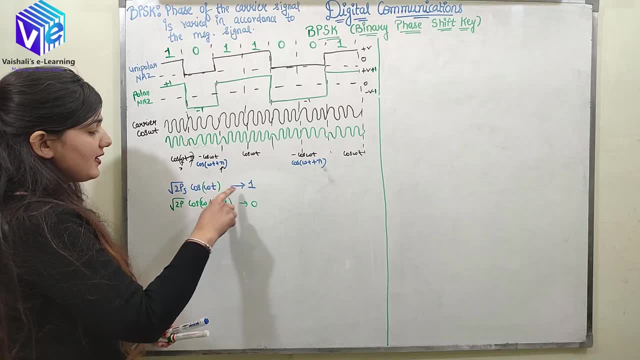 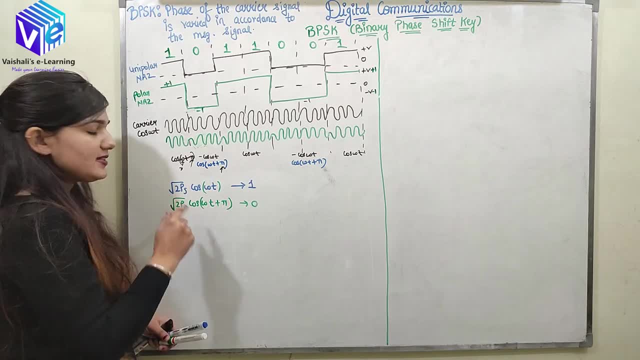 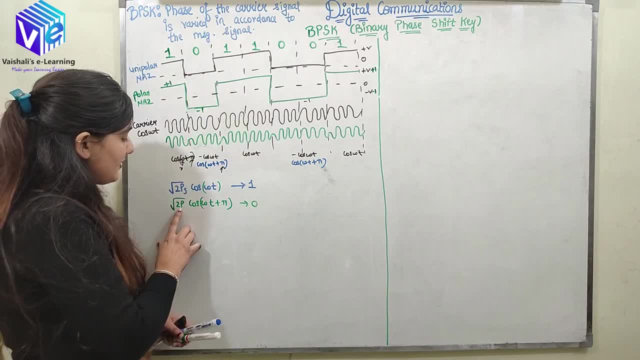 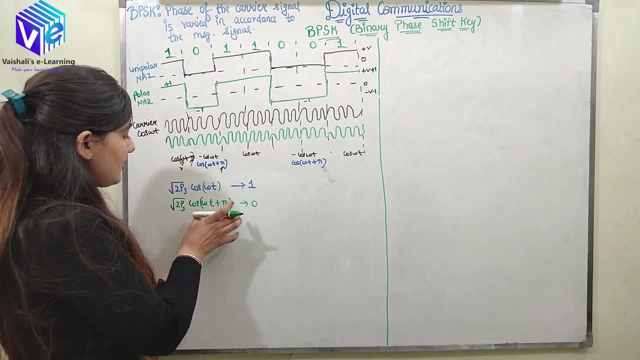 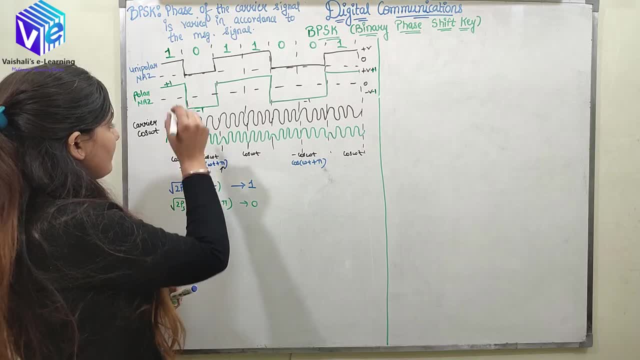 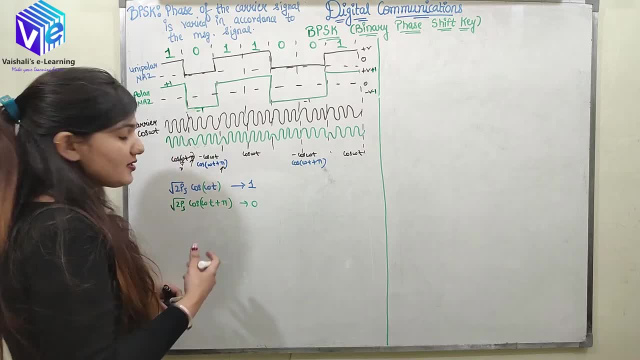 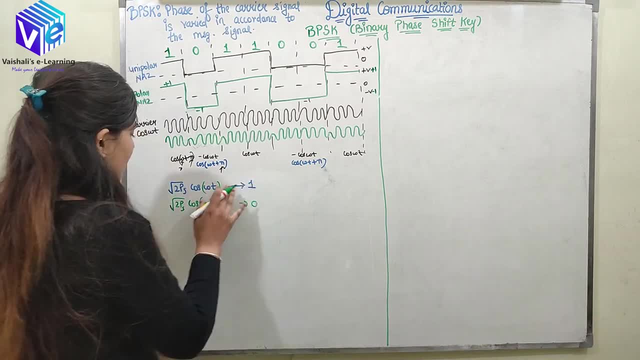 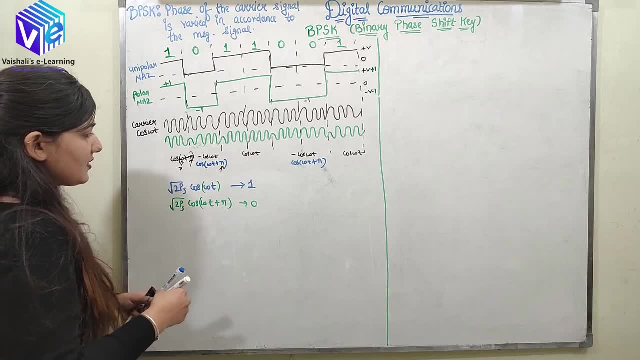 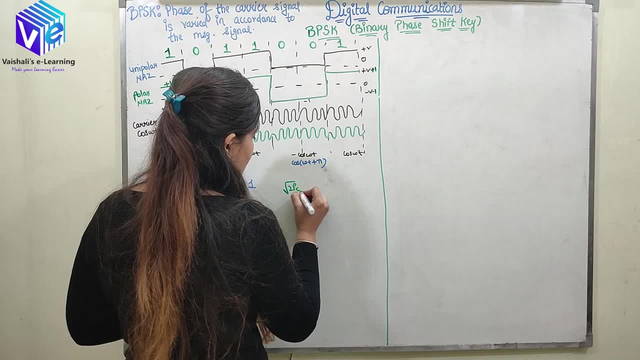 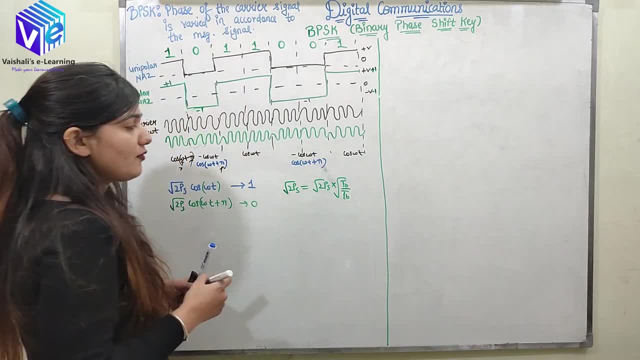 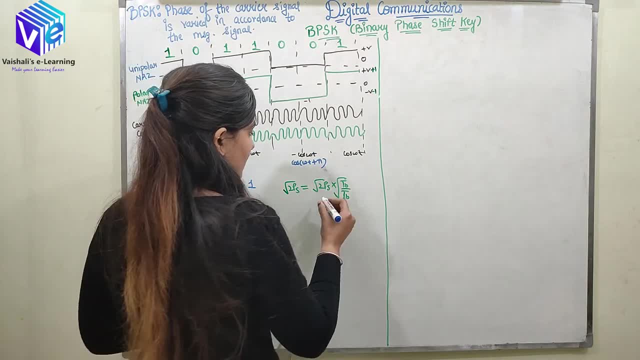 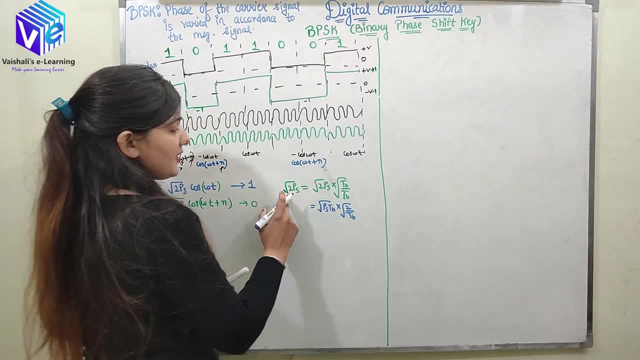 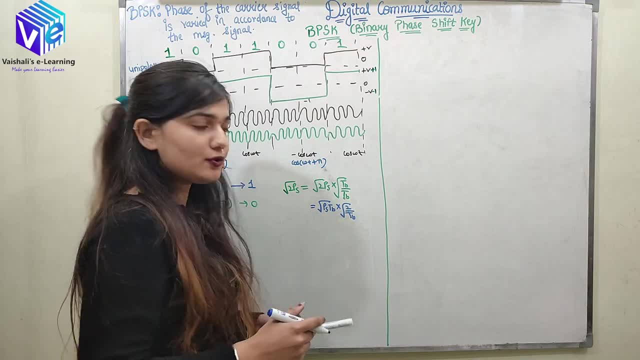 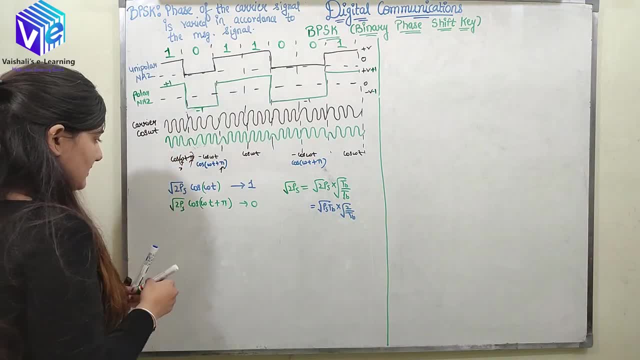 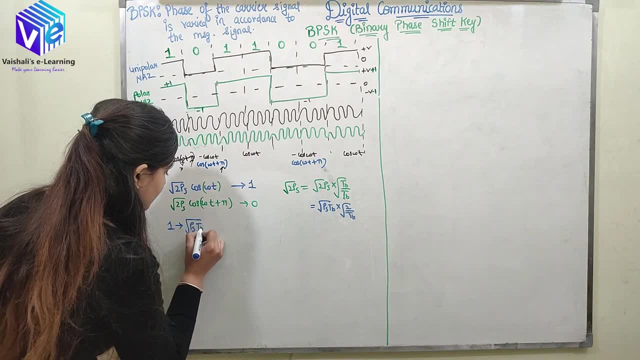 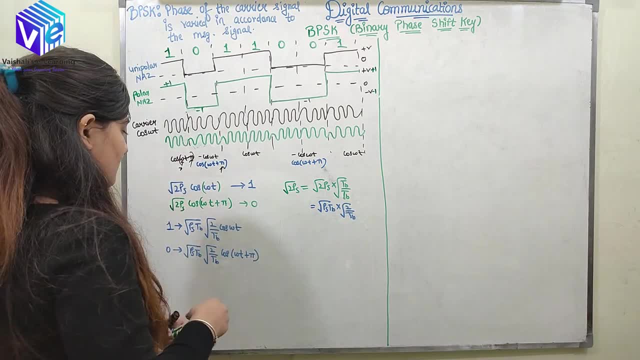 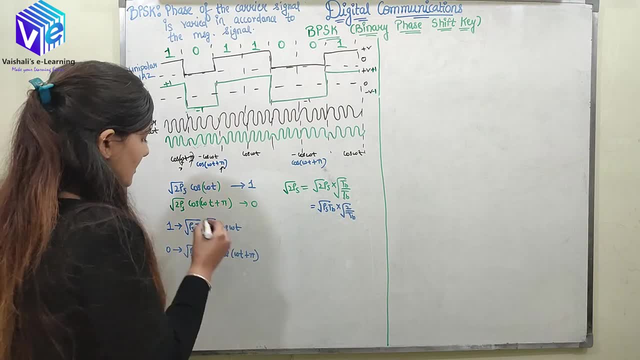 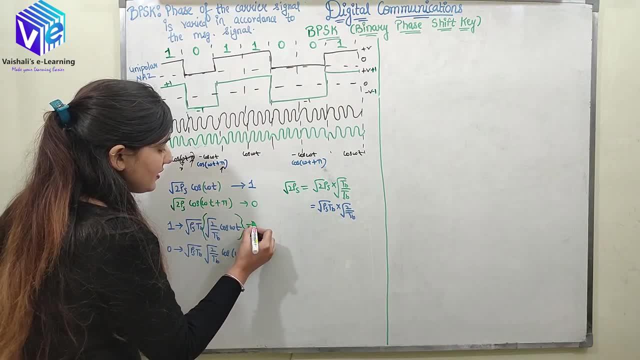 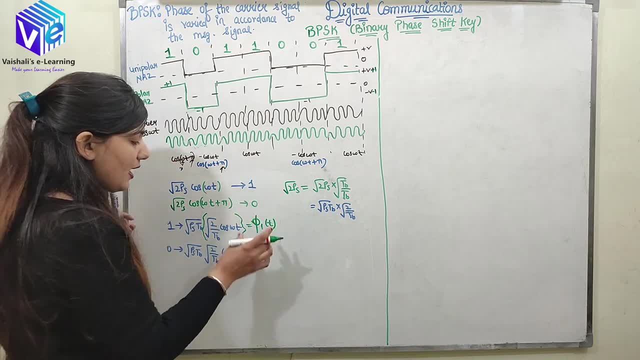 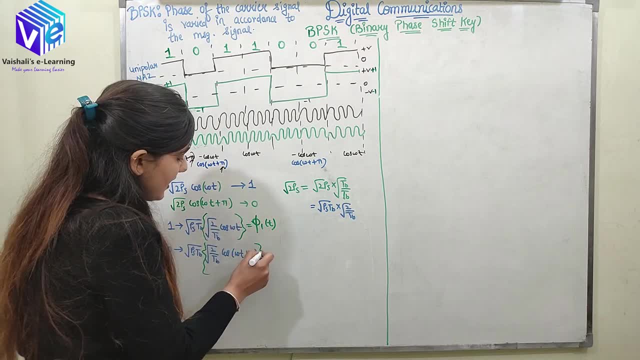 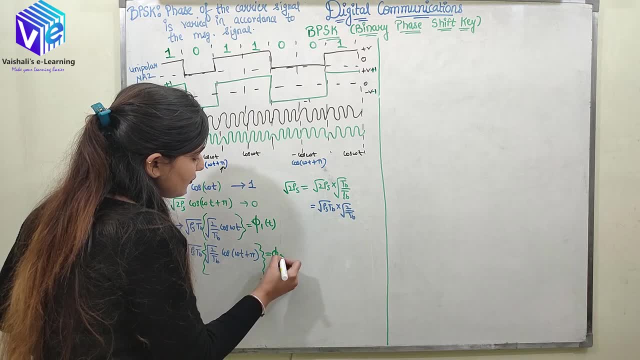 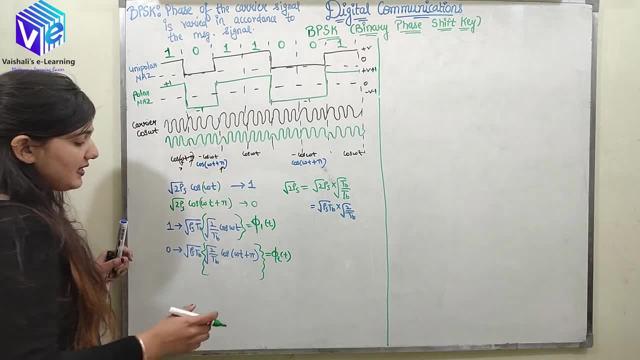 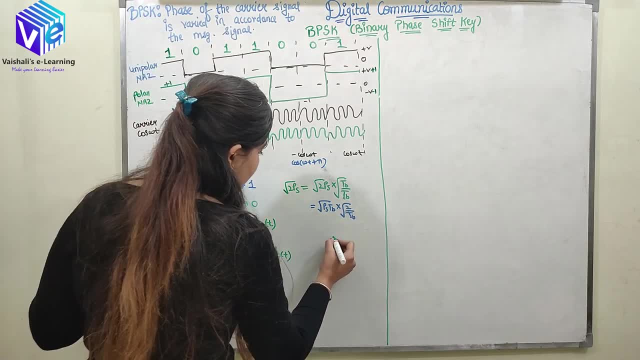 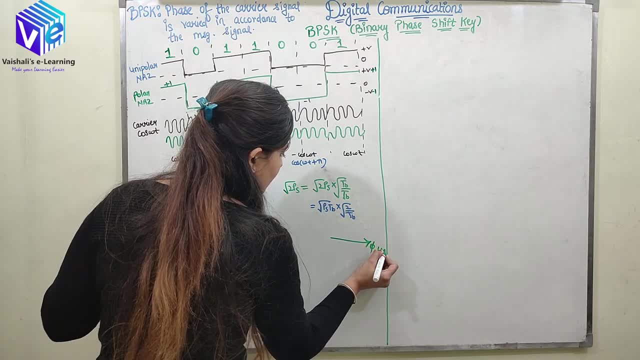 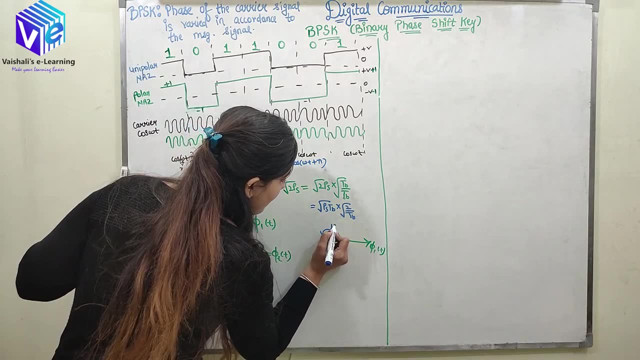 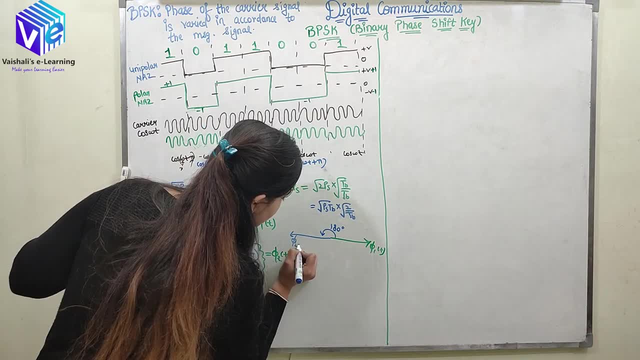 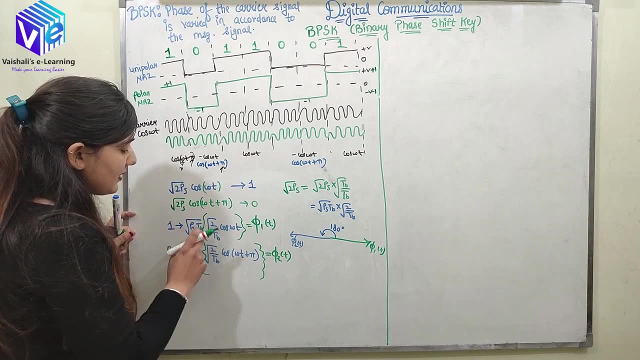 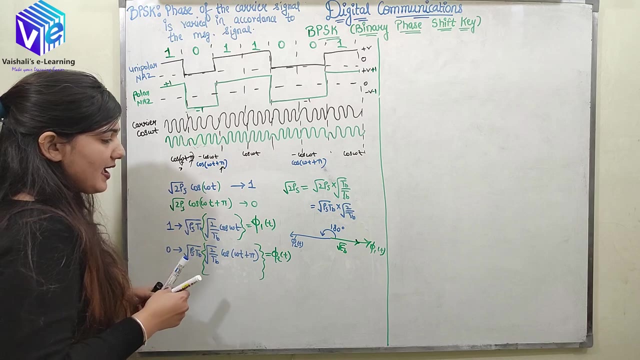 1t, So I can represent my 5, 2t as this. So if I have to make the signal space diagram, so if I project this one on 5, 1t, I will get under root eb or under root ps-tb, which represents my energy. so here also I will get. 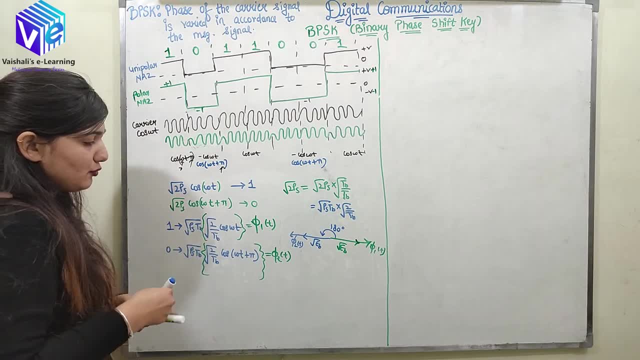 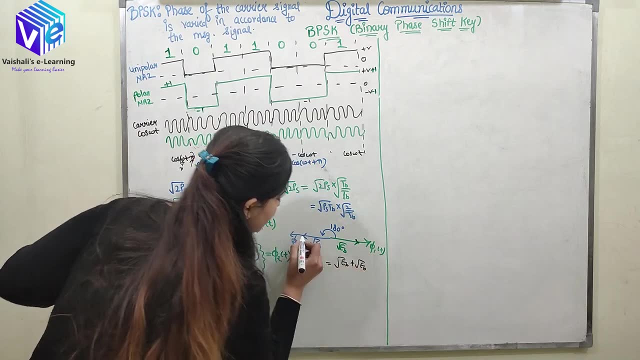 underroot eb or under root ps-tb, which represents my energy. so here also I will get underroot root EB, So D12.. So if here I need to find out D12.. So D12 is equal to, So the total distance. 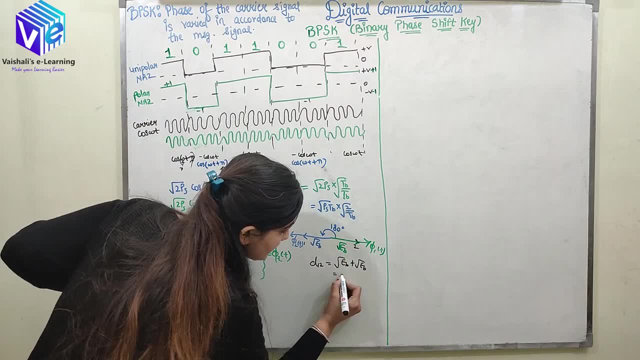 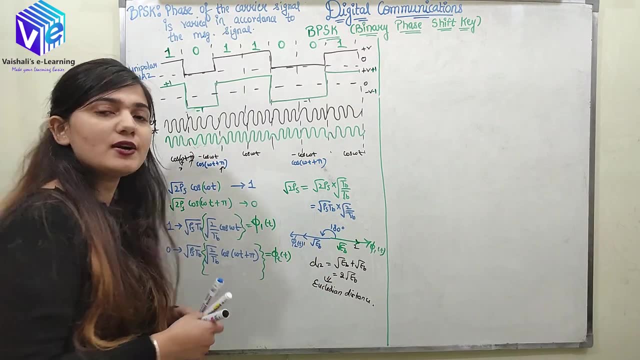 between 1 and 2 is under root EB. plus under root EB is equal to 2 under root EB. So from here I can see that Euclidean distance is 2 under root EB, which is more than FSK and ASK. So now coming to. 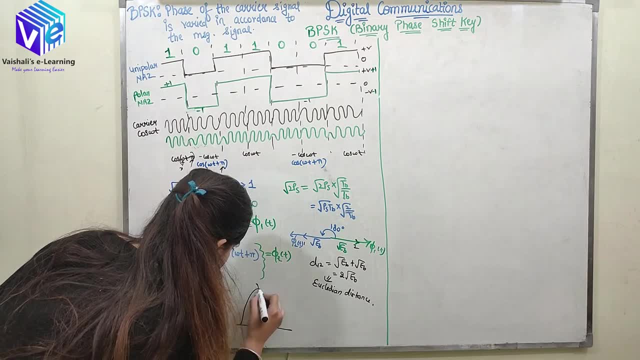 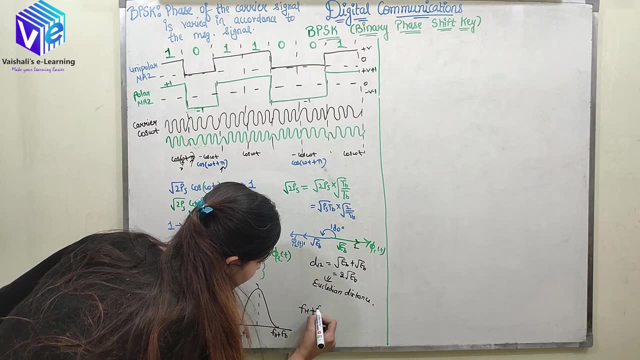 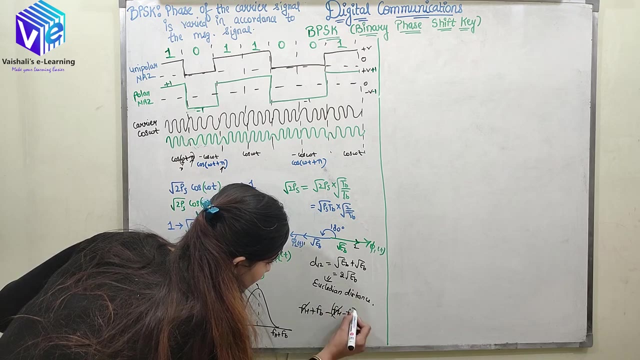 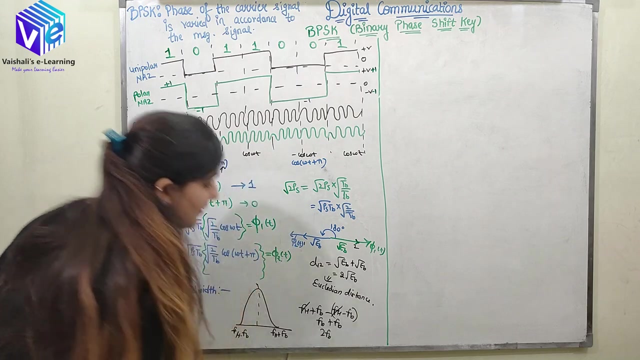 the bandwidth. So bandwidth is high minus low, which is FH plus FB minus, FH minus FB, So minus FB. So FB plus FB minus and minus get plus, So 2FB. So bandwidth is 2FB again, which is equal. 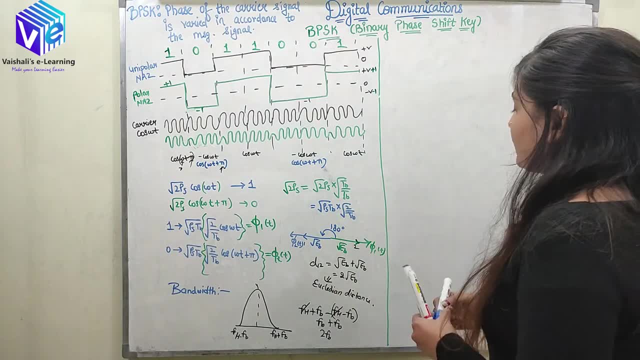 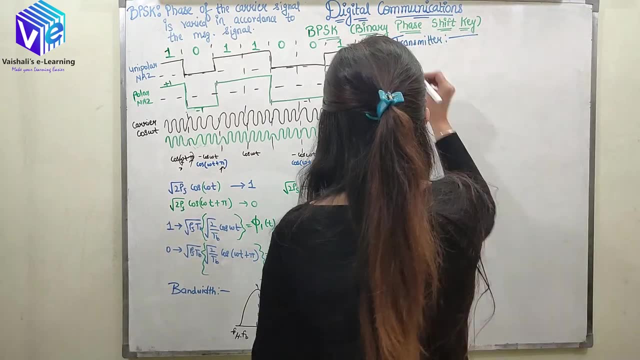 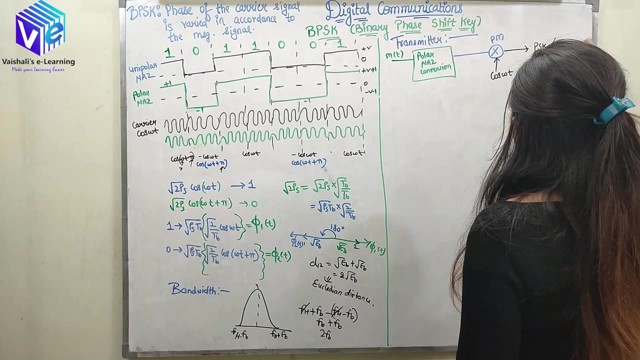 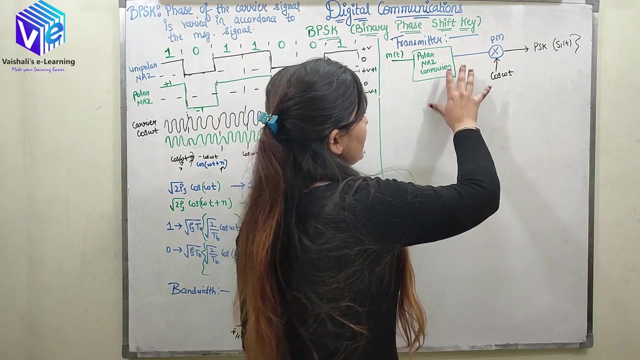 to ASK. So we will compare this as well With ASK. So now, coming to the block diagram of the transmitter. So MT is my message signal which is converted to polar NRZ form. So after it is converted to: 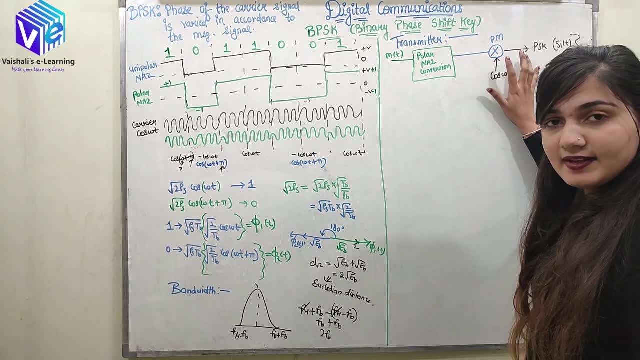 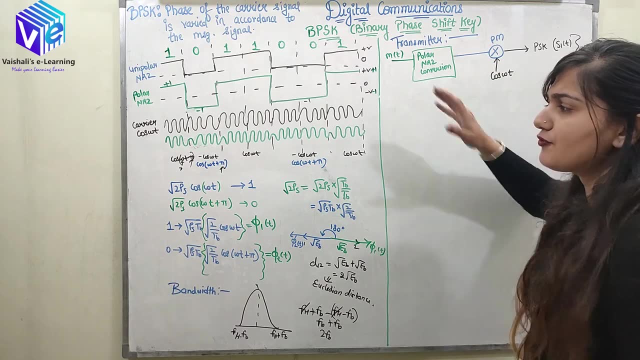 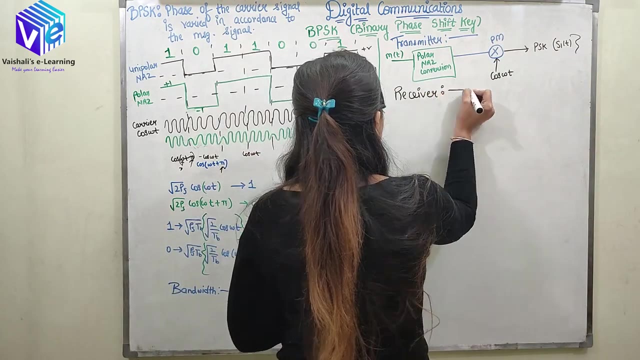 polar NRZ form, it is fed to the product multiplier, where it is multiplied with the frequency carrier and at last I will get the PSK. So from here you can imagine how various blocks are working. So now coming to the receiver. So we have two types of receiver. 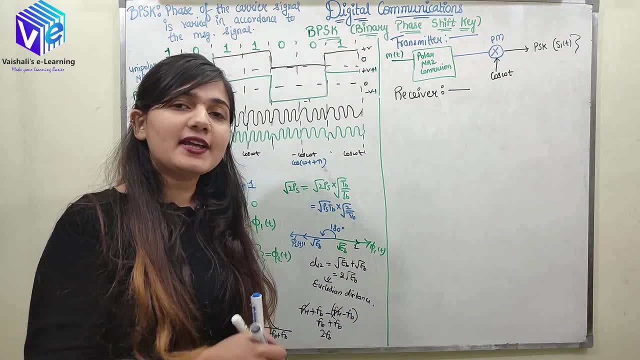 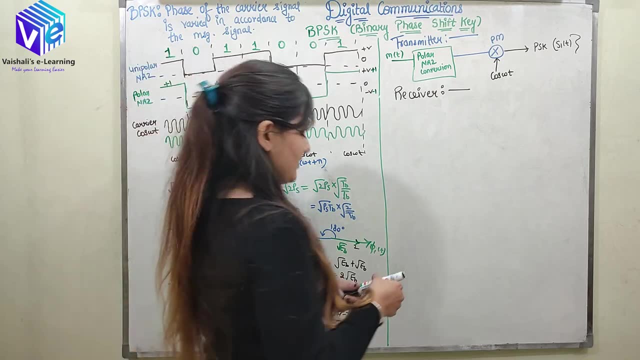 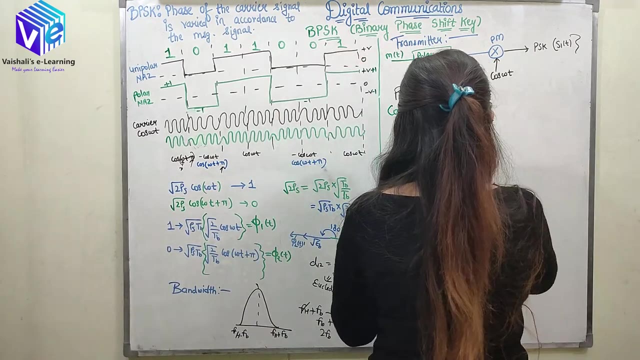 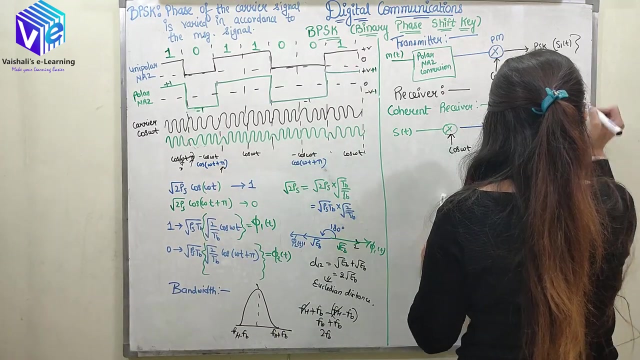 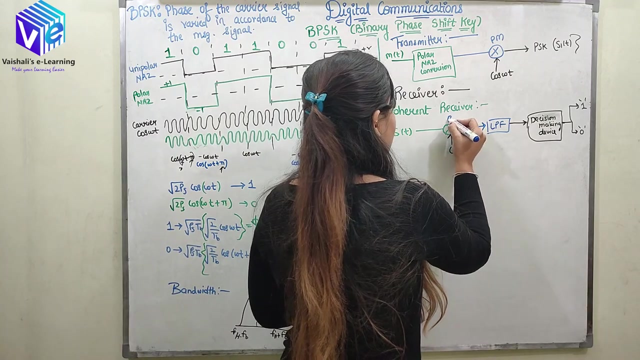 coherent and non-coherent. We will see if we can detect the PSK signal with the help of coherent and non-coherent, both or not. So first we will see the coherent receiver. So now, ST is my modulated PSK signal which is fed to a product modulator where it is. 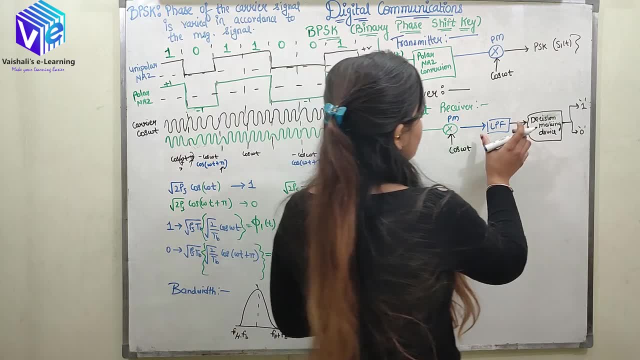 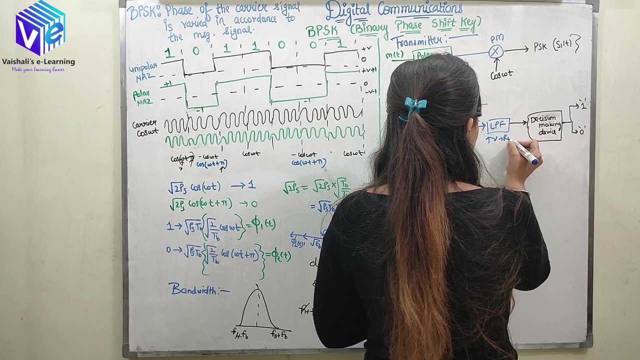 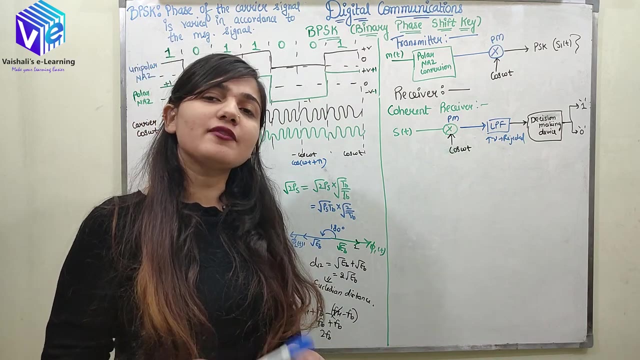 ST is multiplied by cos, omega, t, So, which is passed to the low pass filter, where all the high frequency components are rejected. Then it is passed to the decisionmaking device, where it makes the decision that it is getting 1 or 0. so, in accordance to the 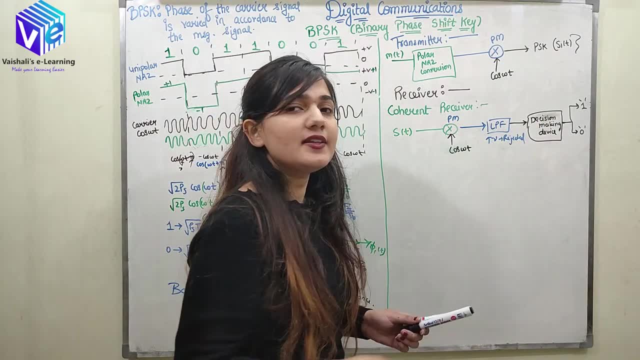 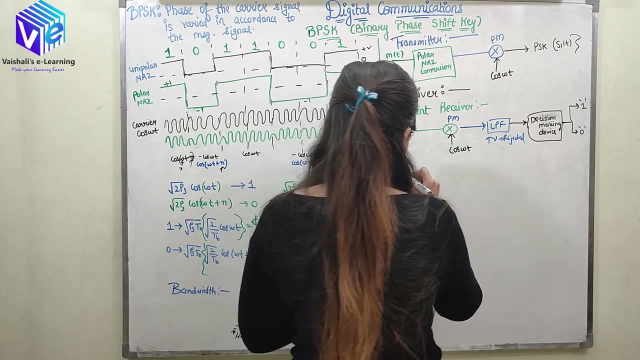 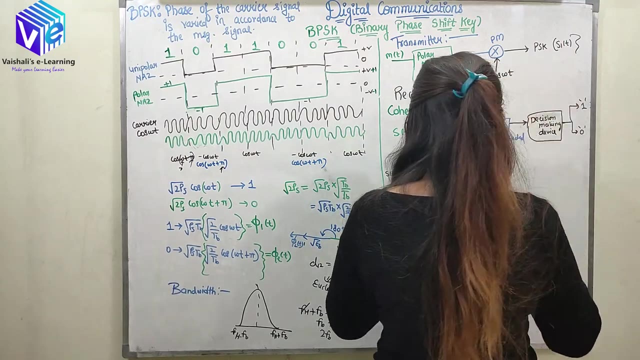 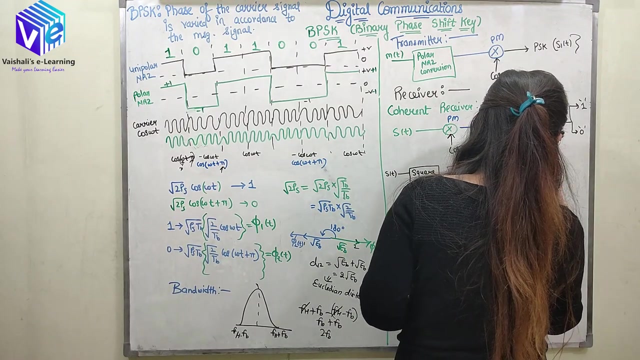 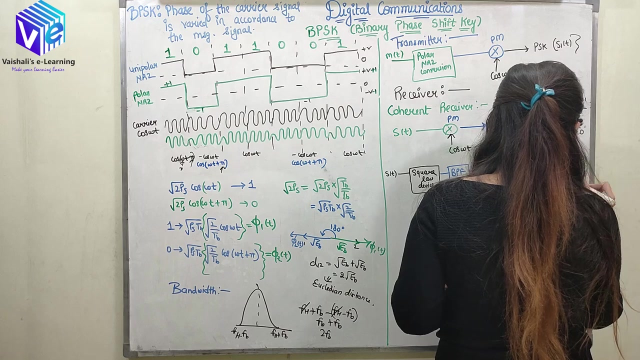 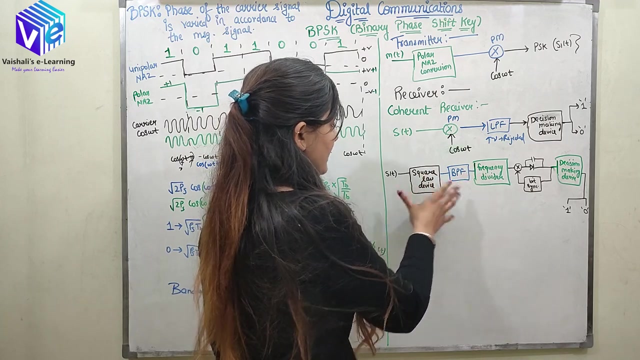 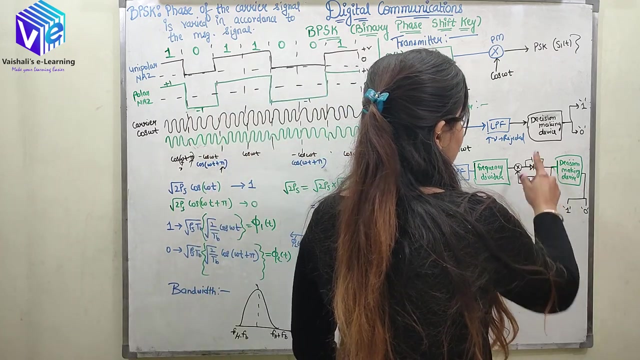 decision made by the decision-making device, the signal is regenerated with the help of regenerator. so now, when I see the current receiver closely? so now, if I see the current receiver closely, it looks like this: so it has a square low device. then after that, bandpass filter, frequency divider, after that, this is the integrator. 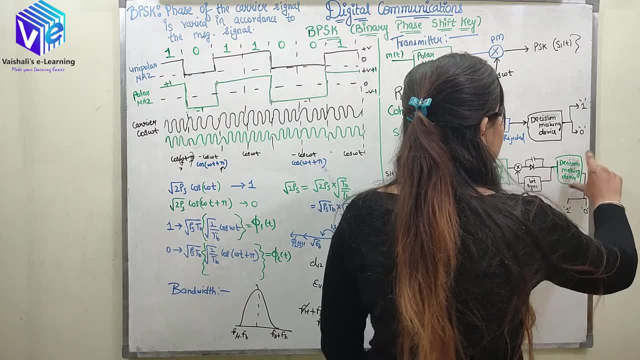 and this is bit synchronizer. after that it is fed to the decision-making device. so let's understand what all is happening in the way it is being made. so let's see the decision-making device. so let's understand what all is happening in the way it is being made. so let's see the 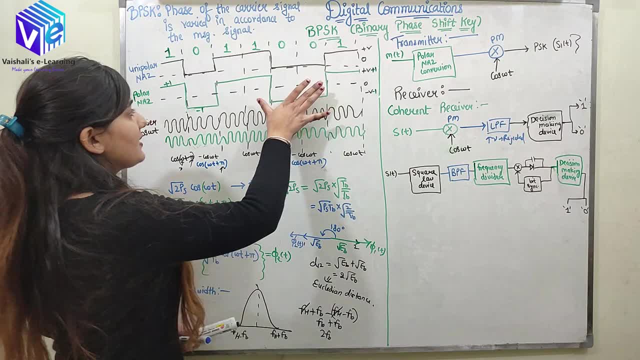 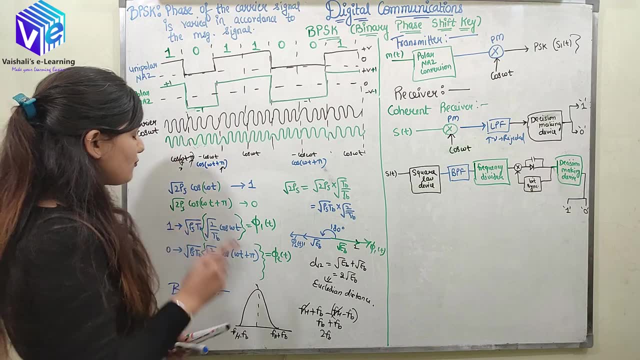 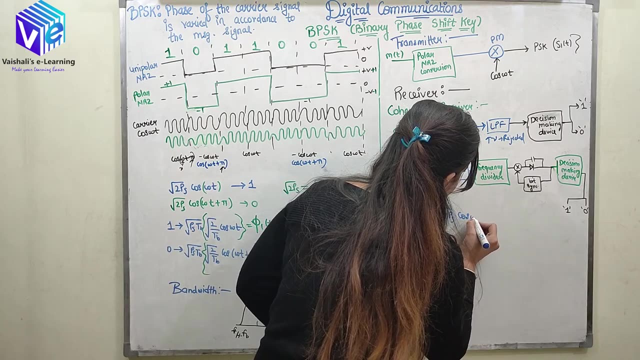 block. so square low device is converting the negative part into positive part only. so if I have the 0, which is represented by minus 2 PS cos Omega T. so 0 was represented by minus under root 2 PS cos Omega T, so it is converted to 2 PS cos square Omega T with. 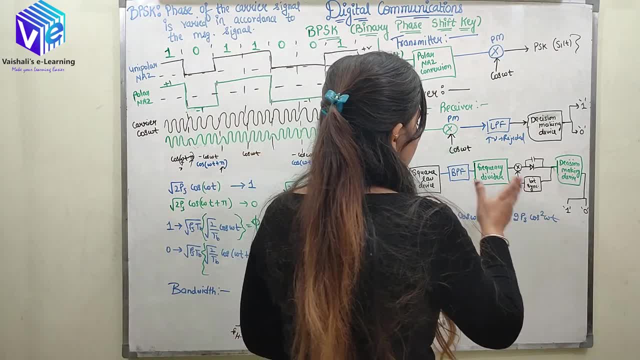 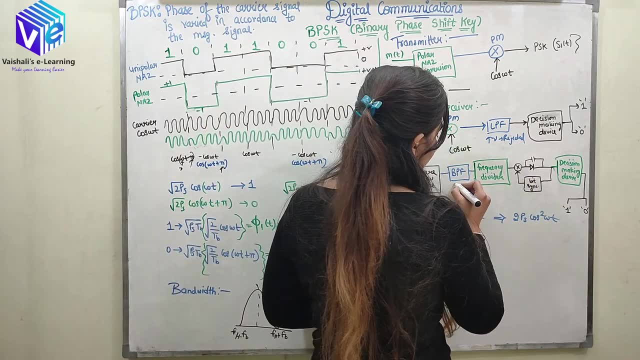 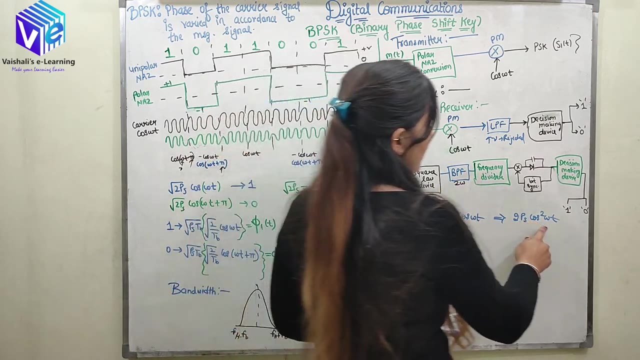 the help of square low device. so square low device is helping me to convert the negative signal into positive counter part. after that I have bandpass filter of frequency 2 Omega, so it is accepting all the frequencies of 2 Omega. so here I can represent my cos as 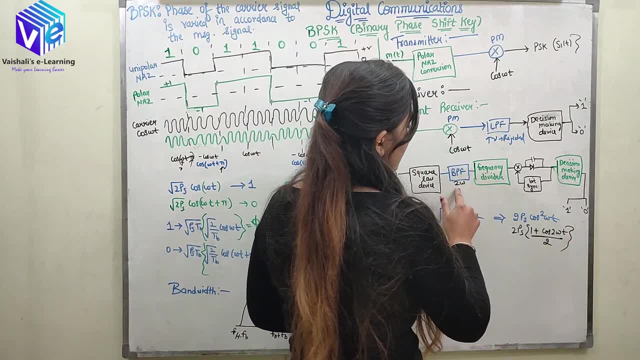 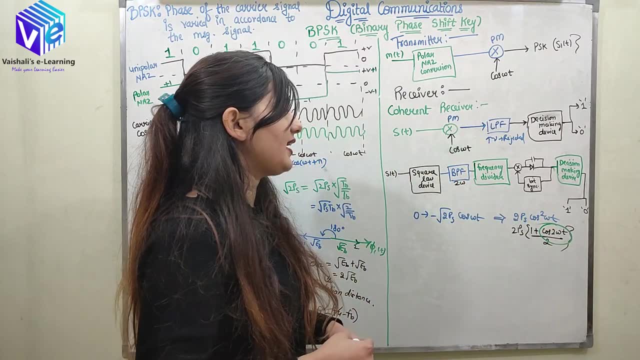 so now in from this signal. the bandpass filter is allowing only this signal, so only this signal is passed after this bandpass filter. after that I have frequency divider. so frequency divider is dividing by a frequency divider. so this is the frequency divider, so this is the frequency divider. 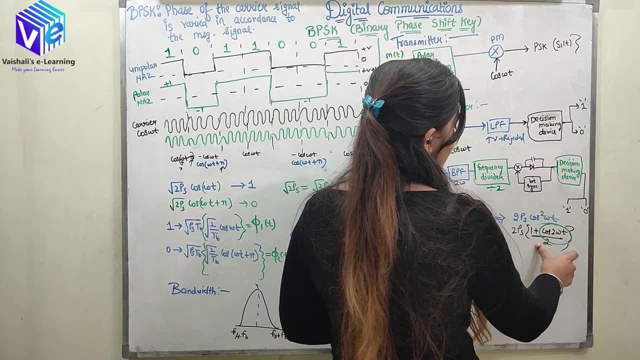 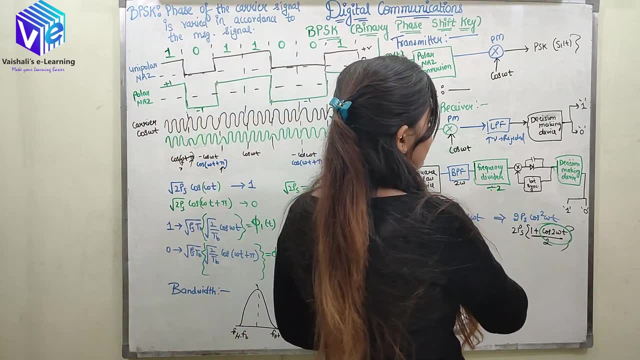 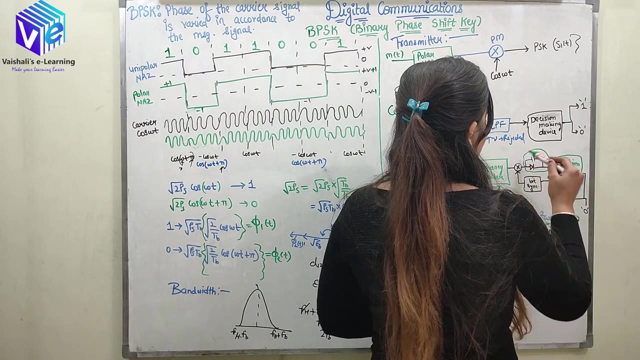 I have frequency 2, so that I had the twice the number of frequencies. so now, after the frequency divider, I am left only with the equal number of frequencies which I fed. so after that I have low pass filter which is acting, which is the integrator, so so after that I have bit synchronizer, bit. 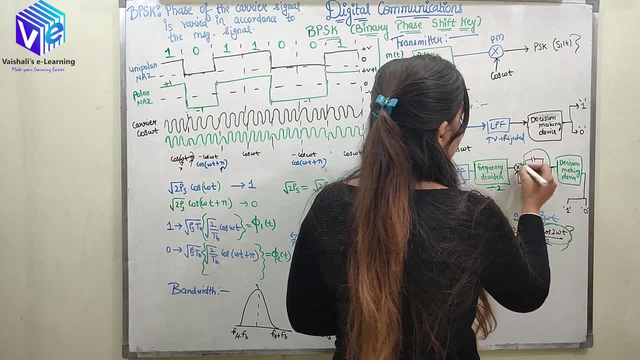 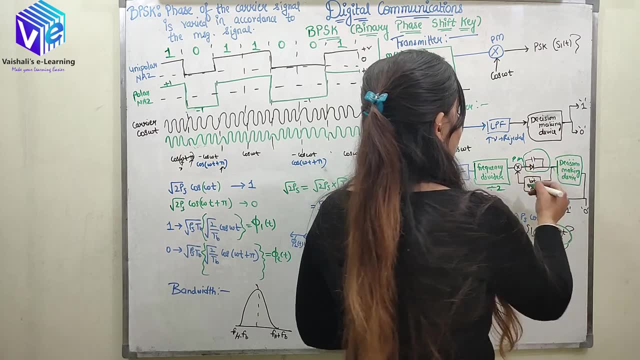 synchronizer is used for the might for the with the help of product multiplier so that the low �� since this video has been extremely informative for the viewers like this, please like, comment, share. integrator can act upon it so with the help of bit synchronizer the product multiplier and the 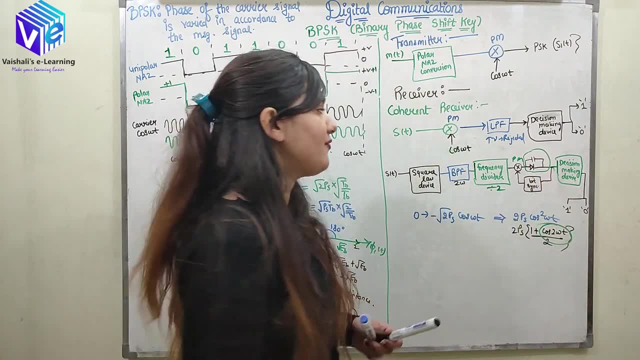 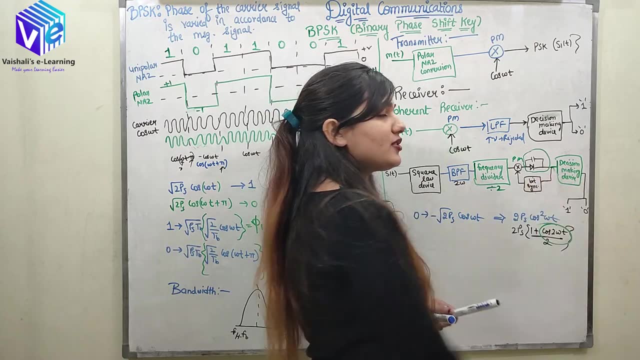 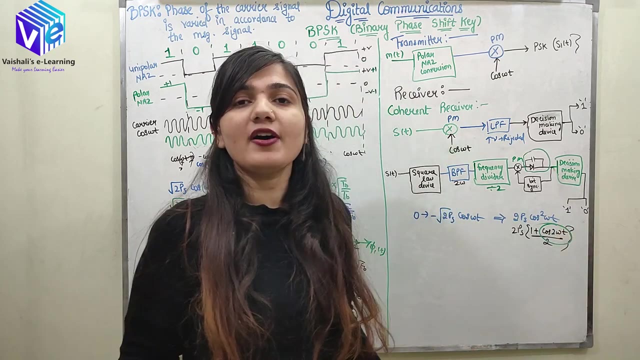 low pass filter is able to reject all the high frequency components. after that, i have the decision making device, which make the decision that it is getting one or zero and, according to the decision it made, it will form a regenerated pulse with the help of the regenerator. so now i